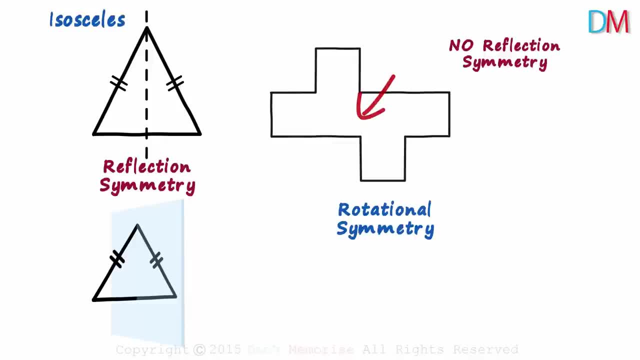 We rotate the figure completely around the centre point once and see how many times it looks exactly like the original one. Rotating it completely means rotating it by 360 degrees. Let's have a counter on the right which counts the number of times the rotated figure looks like the original. 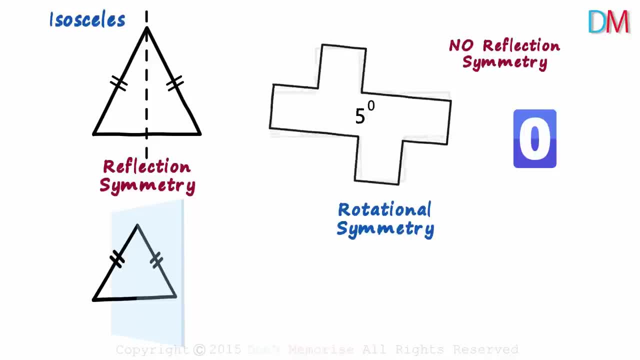 Let's start Now. the figure rests at zero degrees. After rotating it by 90 degrees, we get this shape. It's not the same as the original. The counter is still at zero. Okay, so let's rotate the original shape by 180 degrees. 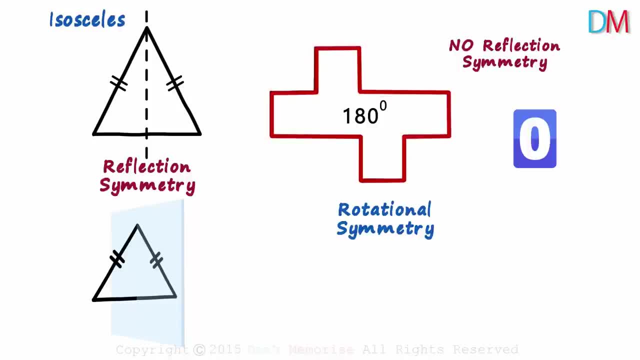 And we see that it looks exactly like the original shape. It fits in perfectly. We see an increment of one on the counter. We continue rotating it till we finish one complete rotation. Rotating it by 270 degrees gives us the shape, which is not the same as the original. 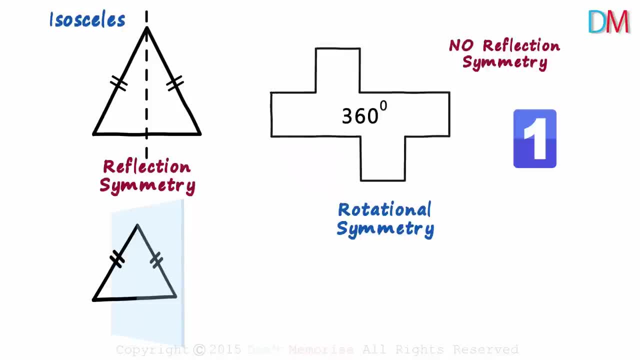 And rotating it by 360 degrees gives us the original shape back, The counter changes to two. What does this do tell us? It tells us that when this figure is rotated completely by 360 degrees, the rotated image looks exactly like the original image twice. 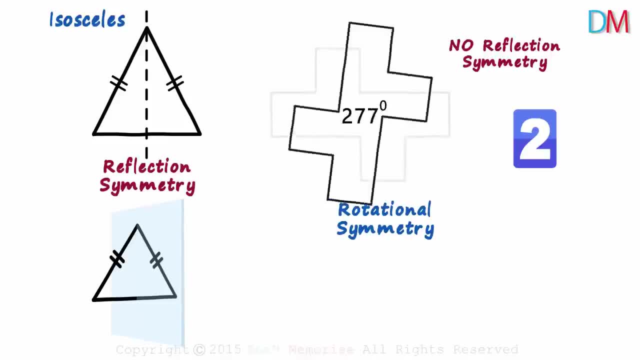 Once at 180 degrees and another at 360 degrees. So we say that this shape has rotational symmetry of order two. To recap, when do we say that a shape has rotational symmetry? Okay, this is long, So I want you to listen to it carefully. 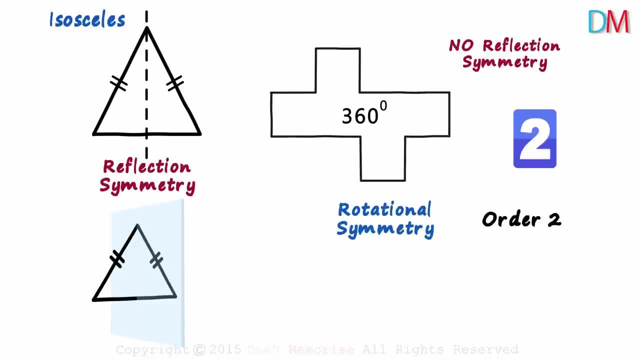 A shape has rotational symmetry if it looks exactly like the original shape a number of times when rotated about the centre point by 360 degrees. Here the number of times it looks like the original is two. So we say that this shape has rotational symmetry of order two. 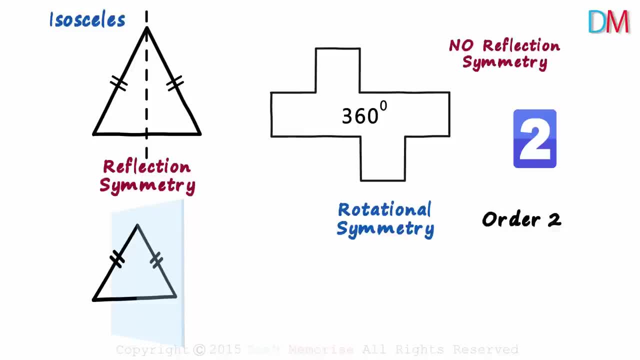 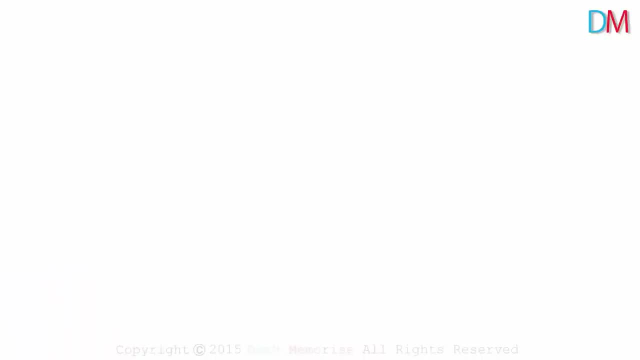 Is it easy to find the order of rotational symmetry? Let me give you a few shapes, and why don't you try finding their order of rotational symmetry? First, an oval looks like this. Next, a square, an equilateral triangle and a circle.